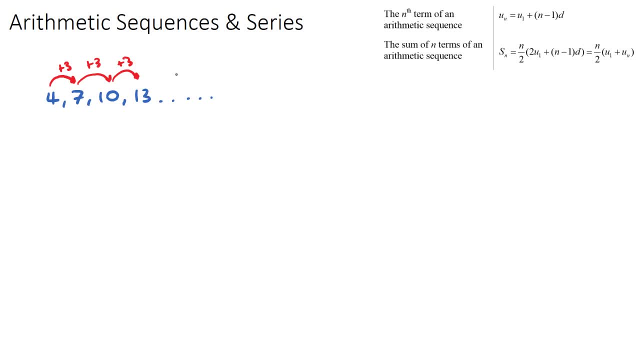 term would be 16 and then 19,. so on, so on. So this is an arithmetic sequence. it's made up of terms and there's a common difference. So there is a letter here, which is D, which we need to denote. 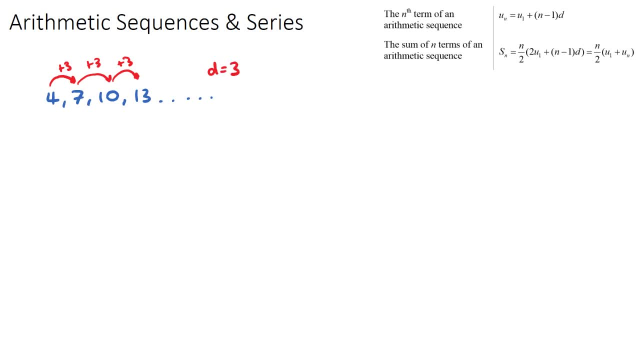 There's our common difference. so in this case, D would be 3,, which is positive 3, and that's going to be important when we use some of our arithmetic sequence formulas. Now I have put the IV formulas up here, which I will show you how these: 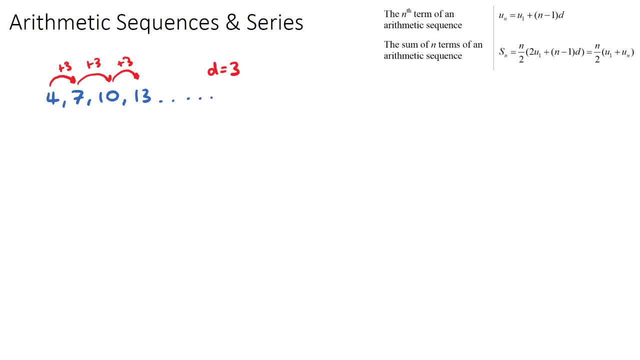 work. Now. another example of an arithmetic sequence is one that goes down. So for example, 20,, 16,, 12,, 8,, dot, dot, dot. This is also an arithmetic sequence, because there is a common difference between these two terms. So for example: 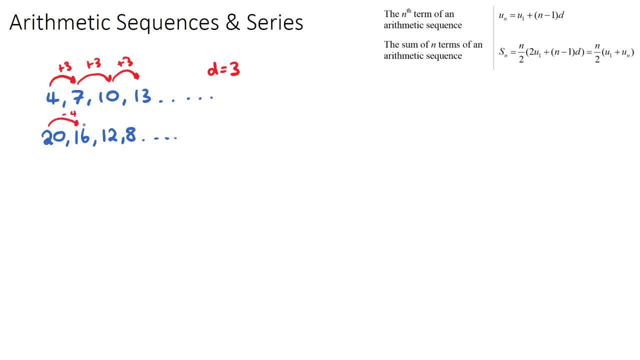 nutrition is a common difference between these terms. now, every white nel in the equation is negative 1 plus 27,. this is also a common difference. Now, I can't be sure if I already said this. there is a common difference, but 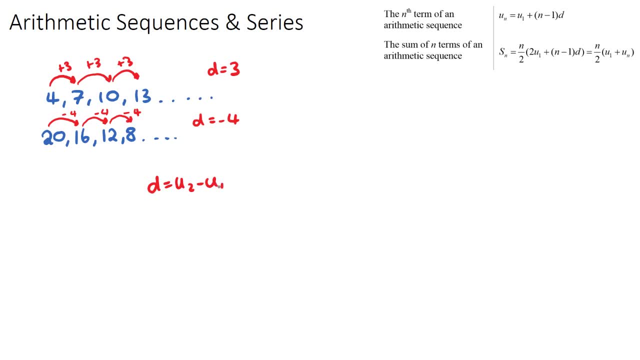 this time it's negative 4, so negative 4, and so on, so on. Now, if it was negative, So u2 means the second term and u1 means the first term in a sequence. So as we can see for this first example that u2, our second term would be 7.. 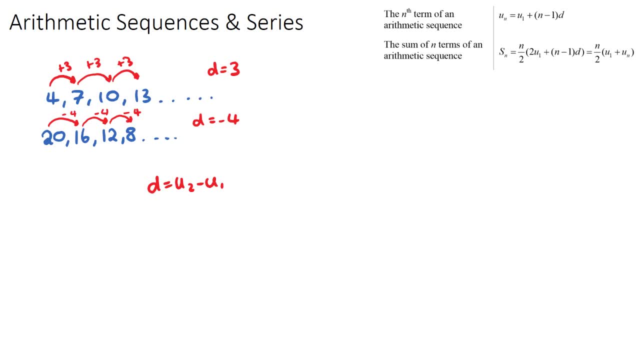 7 minus 4 is our common difference: 3., And this is actually the same as u3 minus u2, and u4 minus u3.. It's any term subtracted the term before it. Okay, so that's what an arithmetic sequence is. 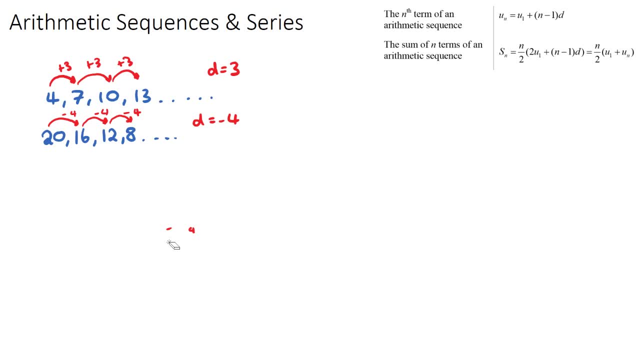 Now, if we have a sequence that has a dot dot, dot, dot dot and it goes forever, this is indicating that it's an infinite sequence. That means it will go on forever. So it could go all the way up to infinity, and then infinity plus 3, and so on, so on, so on. 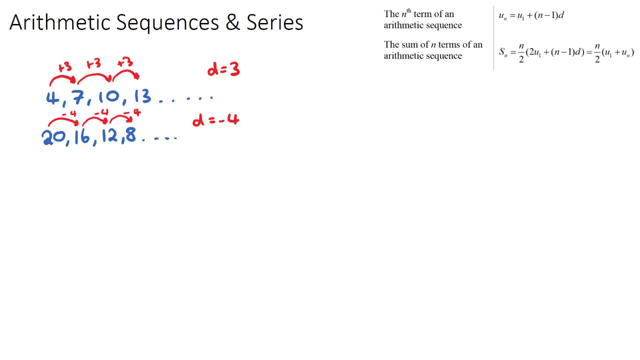 But if we have a sequence that actually stops, so in a question you might have 4,, 7,, 10,, and then dot, dot, dot, dot dot, and then it finishes at 19,. this is actually infinite. 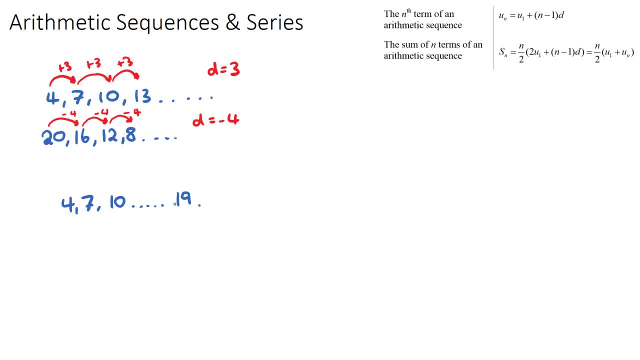 A finite sequence. They've told you that the last term is 19.. So infinite goes forever and finite has an ending term. Okay, so this is what an arithmetic sequence will look like. What we can do is we can use this formula up here to find any term in an arithmetic sequence. 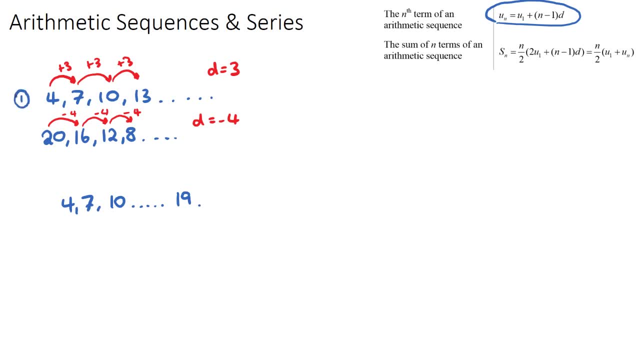 So if we use our example 1 here, if the question asks to find the 100th term, so find u of 100. It would take quite a long time to do it. with your fingers You'd say 4,, 7,, 10,, 13,, 16,, 19,, and it might take you some time. 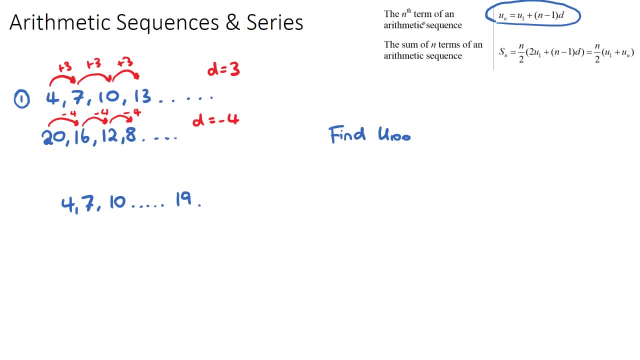 But there is a formula to help us work that out and it's the nth term of an arithmetic sequence. So if we use this formula up here, it says that un- so whatever term we want to find, that's what un stands for- will be the first term plus n, minus 1,. 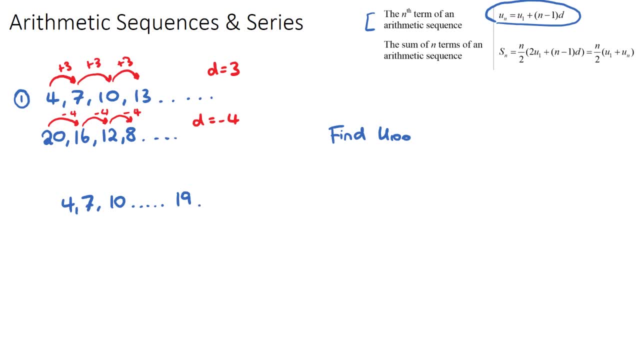 multiplied by, by our common difference. So, using our example up here, if we wanted to find the 100th term, u of 100 will be equal to u1,, which is our first term of 4, plus Now n is the number of terms we want. 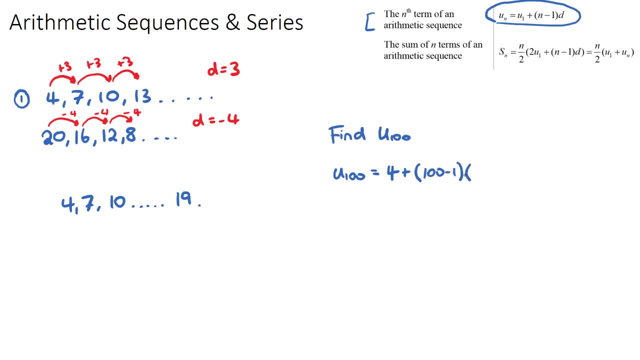 We want 100,, so 100 minus 1.. And we need to multiply this by our common difference, which, for our first example, was 3.. Then we're going to have 4 plus Now, 99 times 3 is 290.. 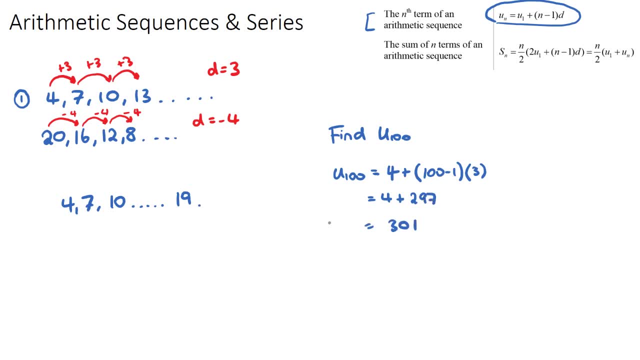 97, so therefore, 301 will be our 100th term. So this is a pretty nice formula. It helps us find terms. Now just be careful: in some IB exam questions They will give you a term in the future. They might give you a term is 301.. 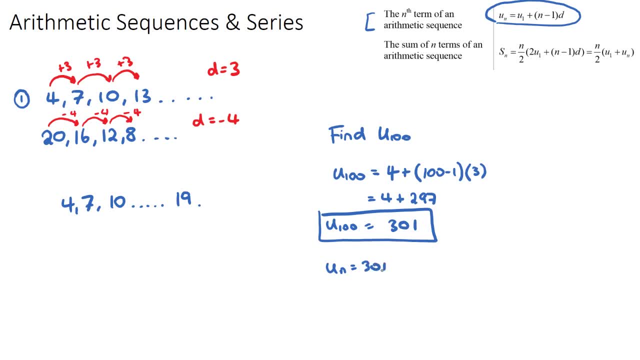 un is 301.. What term is it? So we'd have to let this be 301.. We won't know what n is, But we will know u1 and d, and we might need to use some algebra and work backwards to find that. 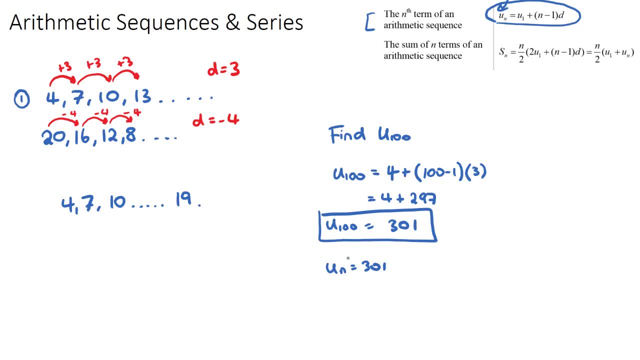 So that's a common IB question. Okay, so that's an arithmetic sequence And an arithmetic series. I'll create some space here. is the sum of a sequence of terms, An arithmetic sequence, So an arithmetic series is the sum of all of the terms in an arithmetic sequence. 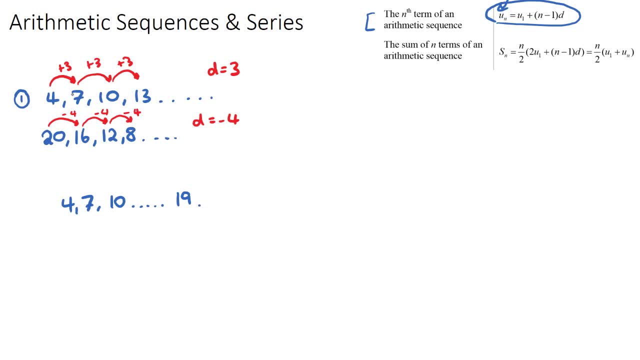 So series stands for sum. So for our example 1 up here, if the question said: if we find the sum of the first, let's say, 10 terms, we'd write it as s10.. This means the sum of the first 10 terms. 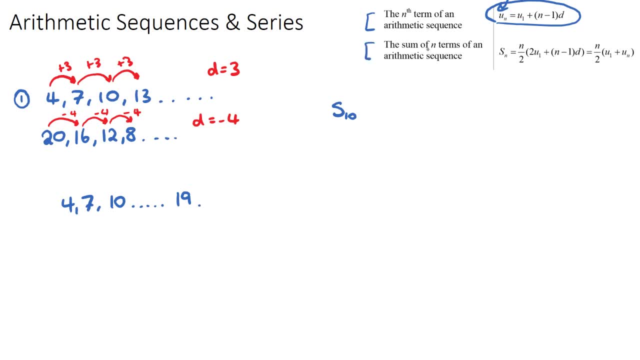 And we can use this second formula here in our formula booklet: the sum of n terms of an arithmetic sequence. So for our example 1, s of 10 will be n on 2.. So n stands for how many terms: 10 on 2.. 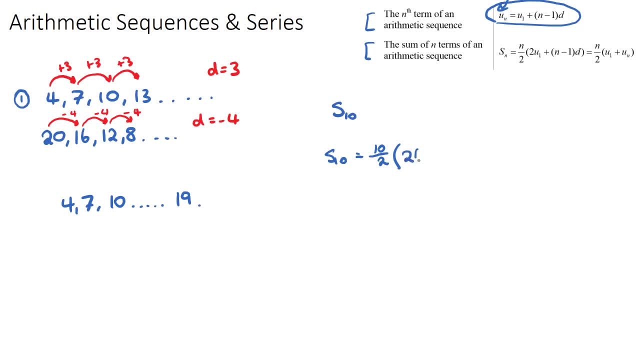 And then 2 times our first term, 2 times 4.. Plus n minus 1.. Well, we want 10 terms. n stands for the number of terms, So 10 minus 1, multiplied by our common difference 3.. 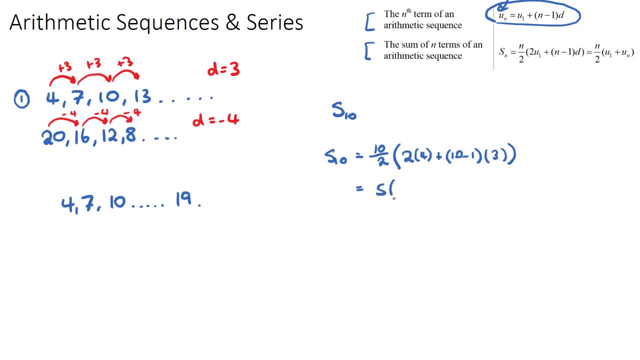 Okay, so we have: 10 over 2 is 5.. 2 times 4 is 8. And 9 times 3 is 27.. Now, 27 plus 8 is 35. And 35 times 5.. We can use our calculator, but it'll be 175.. 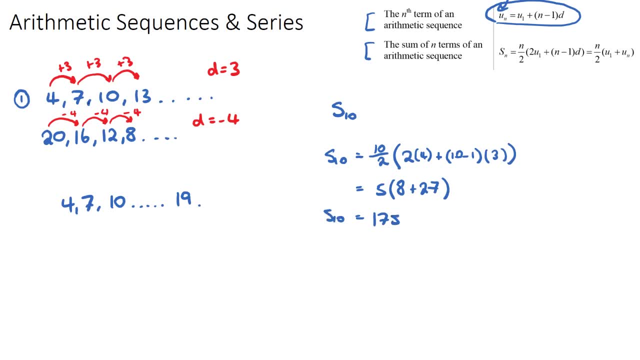 So this tells us that if we summed up the first 10 terms in this sequence, it will equal 175.. Now, once again, they might give you a difficult question where they give you the sum. The sum of n amount of terms is 175.. 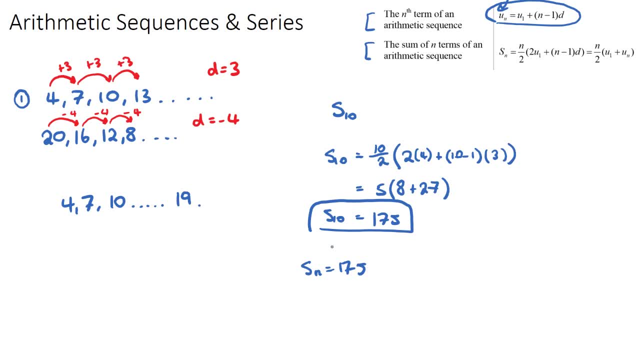 You need to work backwards to find out what n is And, similar to my other example, you just need to put in everything that you know and you might need to use some algebra to work backwards. Okay now, last thing I wanted to touch on is this formula here: 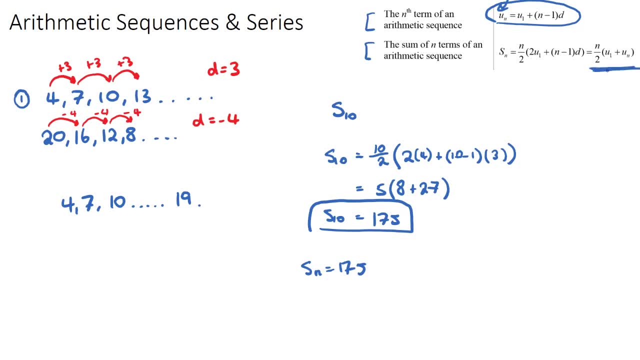 This is also the sum of n terms in an arithmetic sequence, So you could either use this one here or this one, And we can use this little shortcut formula if we have the last term in the sequence. Now, what I mean by that is if the question says: 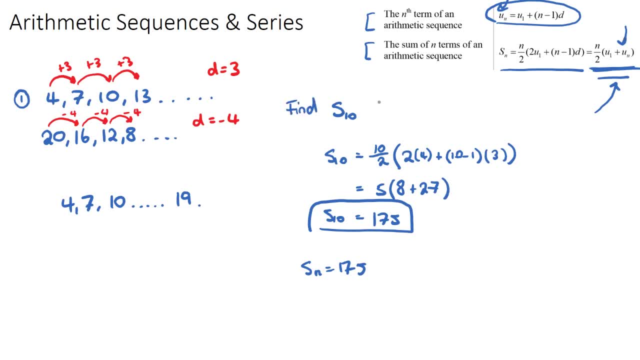 find the sum of the first 10 terms, and we know already the 10th term. have a look at this formula. We want to find s of 10.. And if we know u of 10, we can use this shortcut formula to find the sum of the first 10 terms.